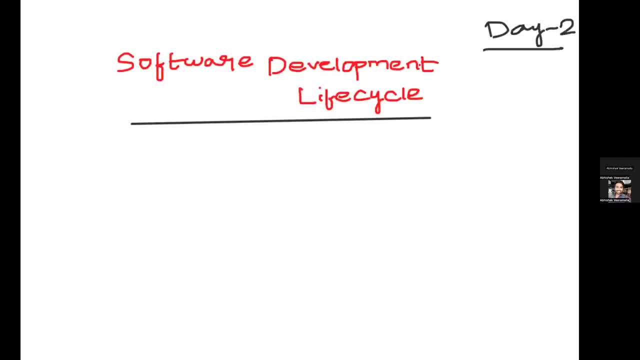 to learn in day two is typically the software development lifecycle. So now you might ask me, like the you know, why do we? why everybody has to learn about software development lifecycle. So, irrespective of the field that you're in, whether you are a developer, whether 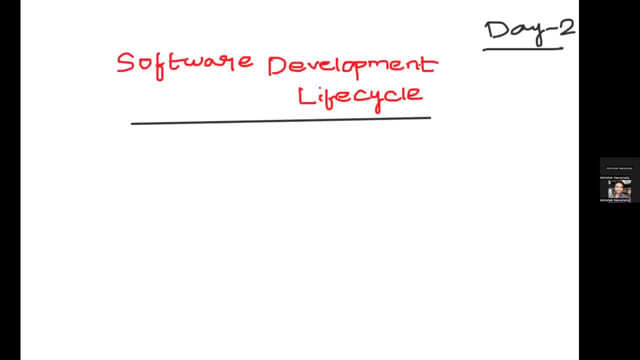 you are a tester, you are into software development or DevOps, everybody has to understand the concept of software development lifecycle. So the software development lifecycle, in short, is also called as SDLC. Okay, so people also call it as SDLC. So don't confuse, don't get confused if 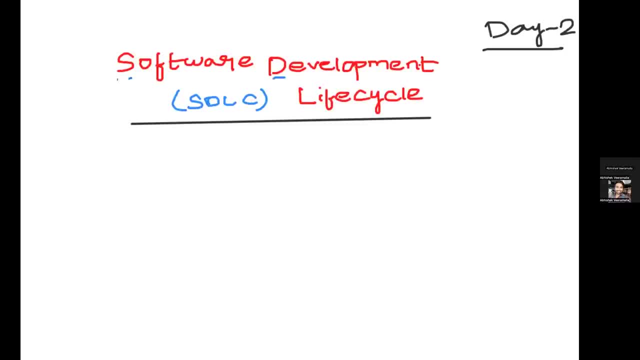 as SDLC. So S D, L C. So this is software development lifecycle. Now, what is software development lifecycle And why is it important for DevOps and all the other engineers to learn this? Okay, so now understand it in this way. We have, you know, opted for a separate and complete day. 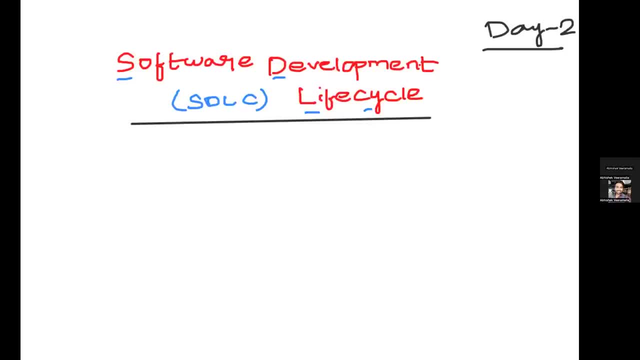 for learning software development lifecycle. That is because everybody has to understand software development lifecycle. If you have a software development lifecycle, you have to work in an organization. So when you work in an organization or when you work in the field of software or the IT industry, there is a standard that is followed by every organization, whether 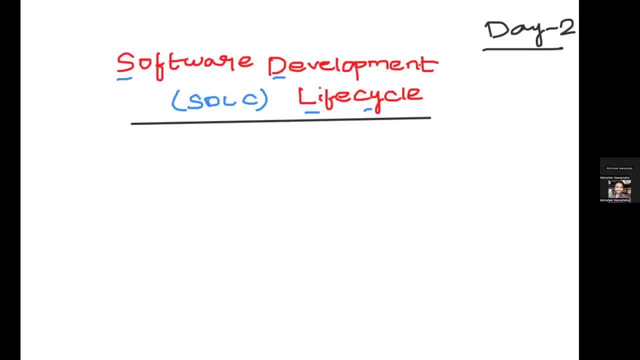 it's a startup, whether it's a MNC or it's a unicorn, everybody follows a specific standards And it is important for you to understand the standards to work in that organization. Now, what is software development lifecycle? it is a process used by the software industry. 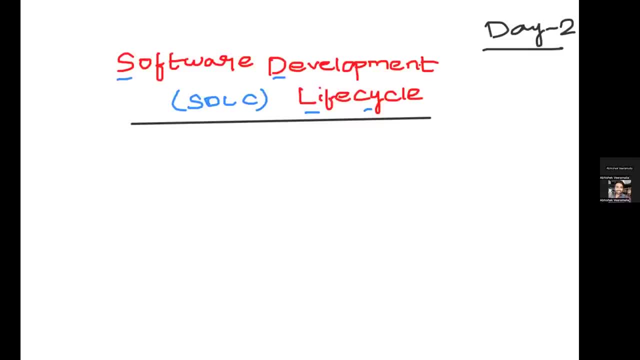 whether it's a process or whether it's again a company or a company with, at the same time, there is a set of standards that are followed in the software industry: to design- Okay- develop and to test, Okay. so to design, develop and test, there is a standard that is followed because 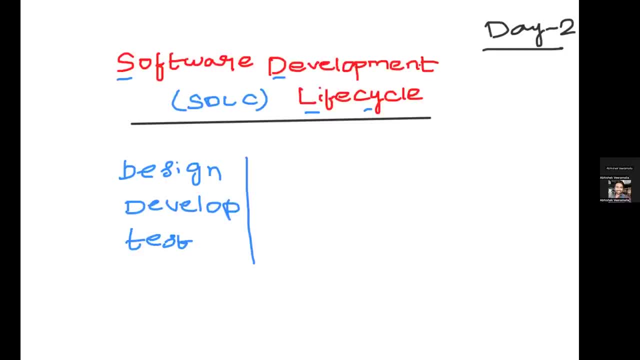 whether you're working at Amazon, whether you're working at flipkart or whether you're working at Tesla. so everybody has to do this. three steps right. One is designed, develop, test, and there are other phases also, but on a high level basis. these are the phases of your 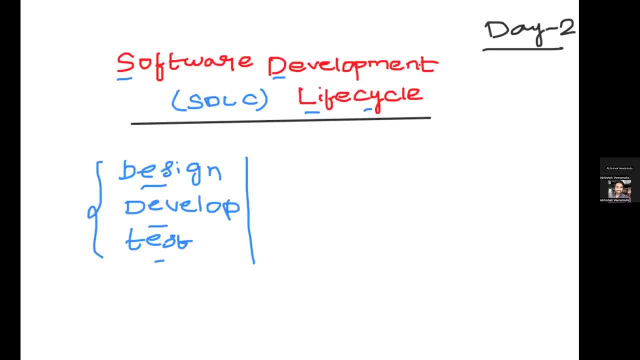 software development life second. now, what are these phases and what are included in each and every of these phase? okay, but before we go there, what is the actual end goal of software development life second? okay, now i said you that there is a design phase, there is a development phase, and 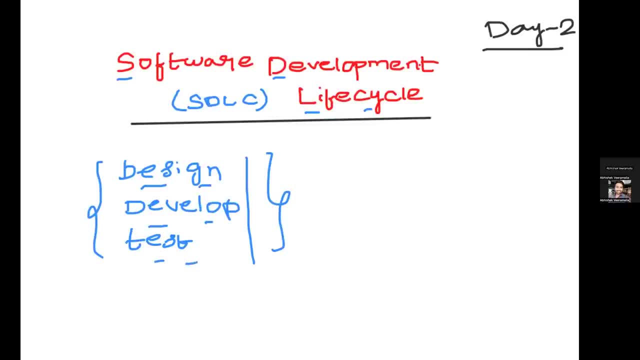 there is a testing phase, but, ideally, what is the end goal? so the end goal is to deliver a high quality product, right? so you might ask me: uh, what happens if i don't test the product? so if you don't test the product? end of the day, you made a design, you developed a design and you delivered it to the customer. 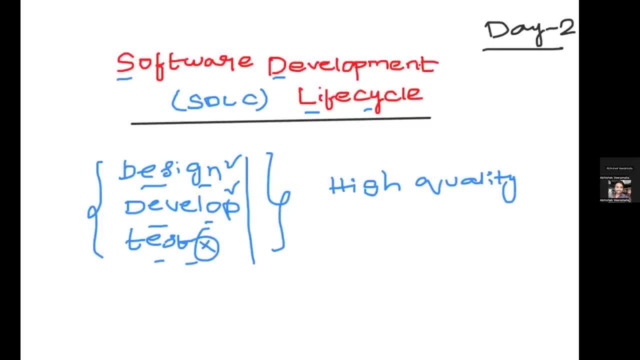 but who was testing this uh product or who was testing this delivery? so that's why, to meet your customer expectations, or, you know, if you want to uh deliver a prompt application to your customer, you have to follow these phases. like without design, you have to follow these phases. like without design, you have to follow these phases. 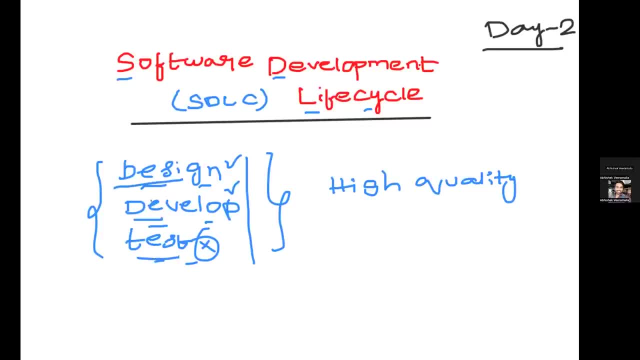 you cannot develop, and once you develop without testing, your product will not be of high quality. so that's why you have to follow the standard to deliver high quality product. so this is a overall high level uh explanation of software development life cycle. that is, software development life. 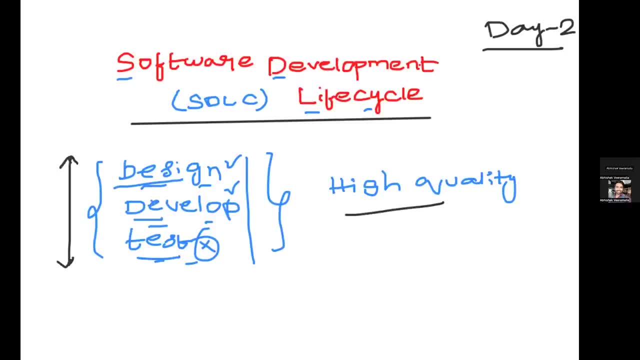 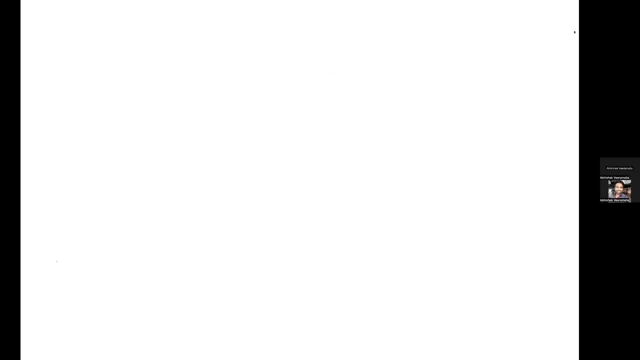 product and we'll try to develop a high quality product and we'll try to develop a high quality. So what I'll do is I'll show you with an example. Let's say we are working at Flipkart, Okay, or to avoid any such names. 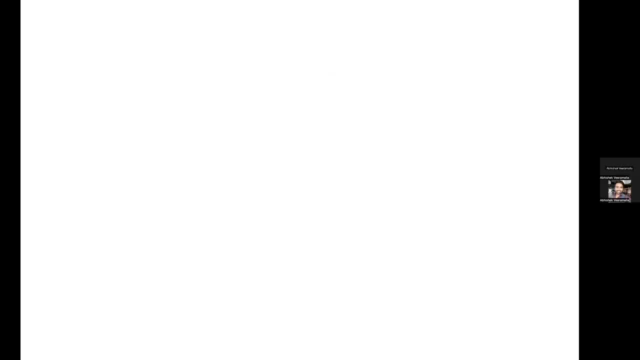 What I'll do is: let's say we are working at examplecom, So examplecom can be any e-commerce website. So let's say I'm working at examplecom, So this can be anything. This can be Flipkart, This can be Amazon or anything. 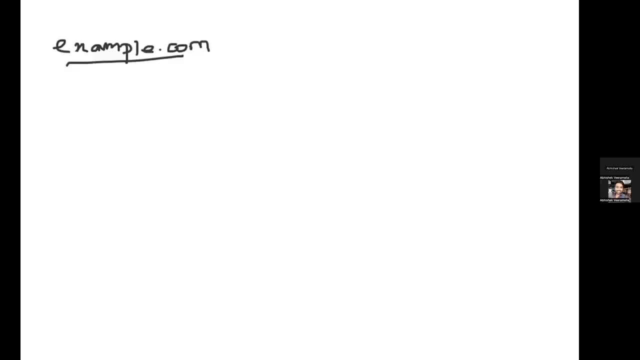 So, for just for our understanding, I just named it as examplecom. So now at examplecom, we deliver a e-commerce application. Okay, let's assume that we are building and developing a e-commerce application. So, again, the process will be same for any organization. 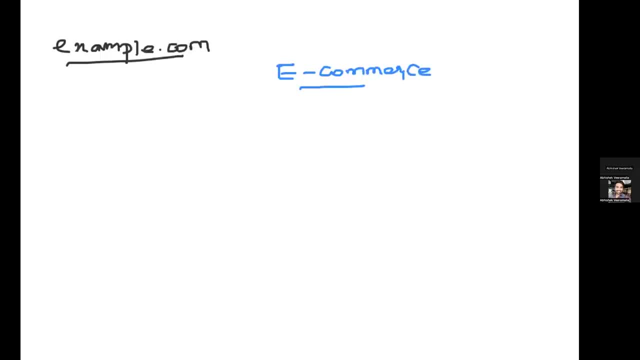 but just for understanding and reference, we are choosing examplecom. So now in examplecom, what usually happens is there are different phases before we deliver the application to the customer. Okay, so these phases are not Nothing, but So you have, let me try to do it in this. 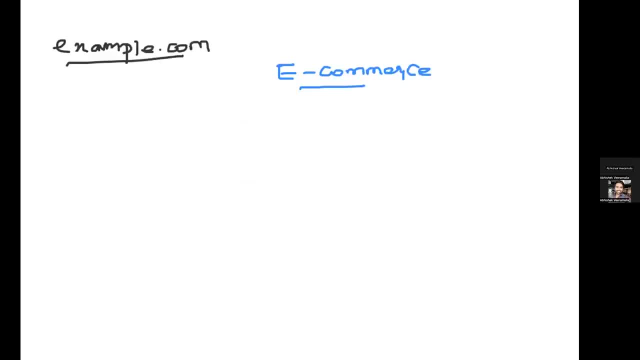 Okay, so we can draw it by ourselves. That's fine. So we have. firstly, we have a phase called planning. Okay, we'll deep dive into each of these things. Okay, don't worry. Then we have a phase called: 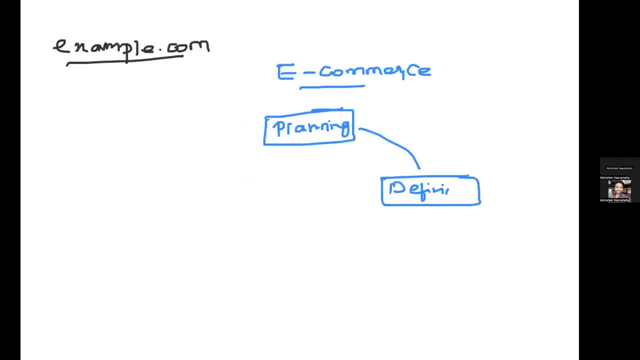 So this is a standard thing. You can refer any book or you can Go through any videos, So these steps are same because there are standards, right, These are called standards. So for standards, everybody has to follow the same standards. So these are standards that are approved and 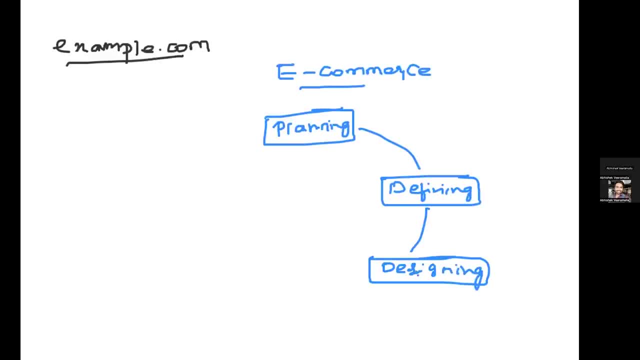 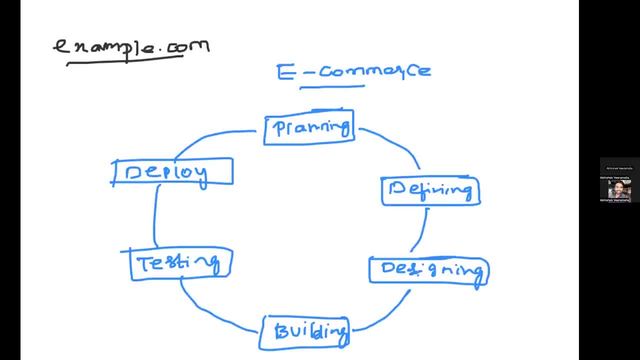 Okay, and then whenever we want a new feature again, we'll follow the same approach. So that's why this is a circle. Okay, what is the reason why I took a circle here? Like you know, I draw a circle here because everybody has to follow this circular approach for each and every feature that they are developing in their organization. 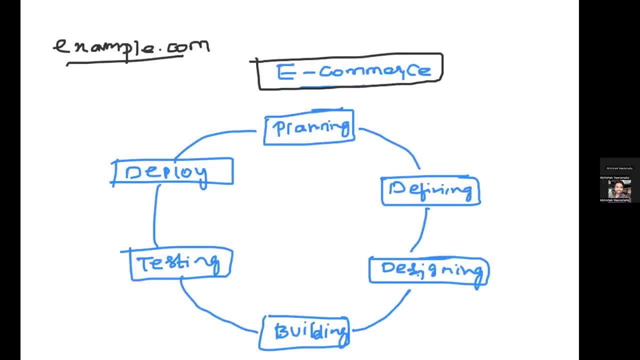 Okay, let's say this ecommercecom Okay, or this examplecom. What they have decided is they want to Start a new feature or they want to support a new feature to the customer. So let's say, just for an example: okay, let's say they don't have kids section. 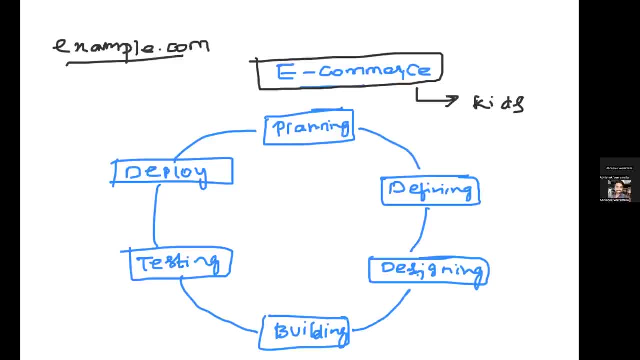 Okay, understand this as a ecommerce merchant or cloth selling website, and this cloth selling website were not selling cloth for kids. Okay, till this point of time, they were only selling for men, Women. Okay, they don't have a kid section. 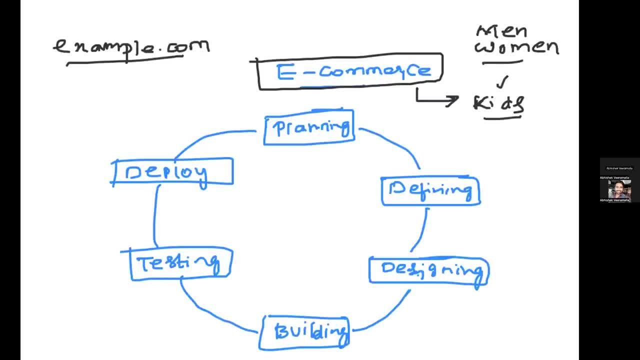 So what the organization has decided Was: on their research, They found out that examplecom can also get benefited from selling kids, kids clothing. So they have decided, like you know, the organization has decided to launch a kids, kids catalog. So for that, what happens is they have to go through this process. 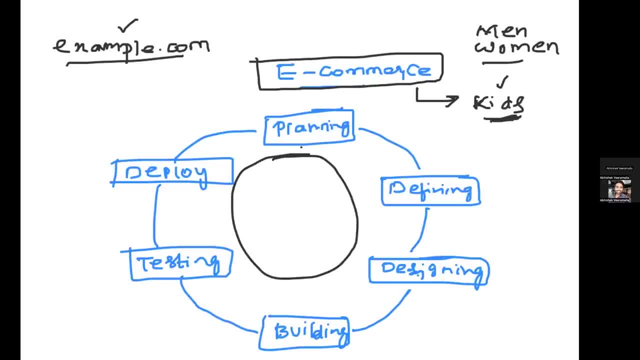 Okay, so this is the standard that is followed across the organizations, Right? So let's try to understand each and every phase. Now, once we understand each and every phase, we'll also Try to see where devops will come into this picture and how can devops improve this process, right? 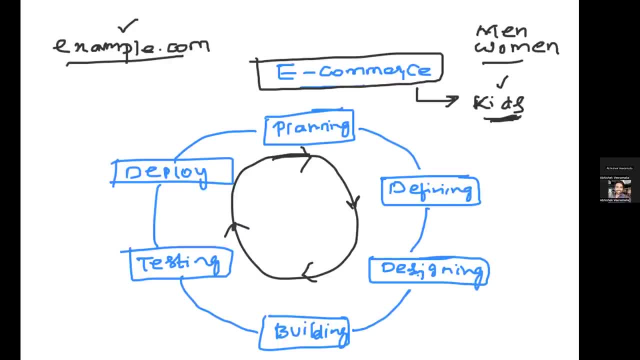 Because our end goal is to understand software development lifecycle and also understand this in the point of view of a devops engineer. Okay, because you have to. once you join an organization, you have to improve your organization's efficiency, right, Your end goal, like on every class that we are learning. only think in a point of view that whenever you are learning a new thing, let's say you're learning terraform. 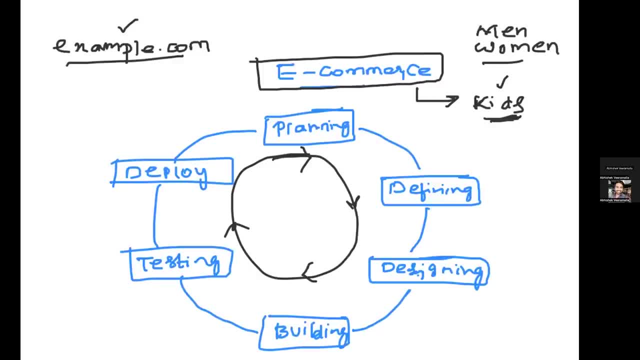 Let's say you're learning ansible. Your point of view, Okay. Your point of view or your way of thinking has to be in a way that: okay, No, I'm learning terraform. How can I use this terraform in the organization and how can I improve organization's efficiency? 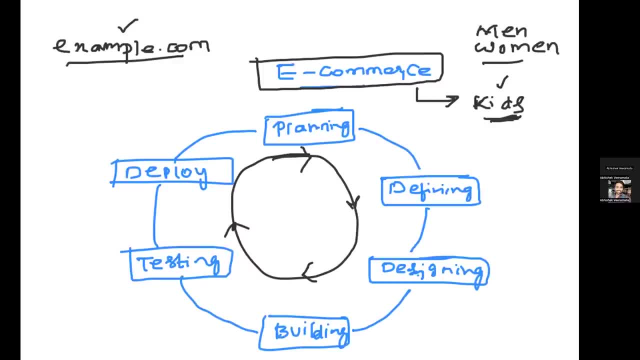 That should be an end goal and you are the member who has to decide if your organization will require this or not. Let's say, everybody in the everybody in the devops community is promoting terraform, but it might be that in your organization terraform is not a right fit. 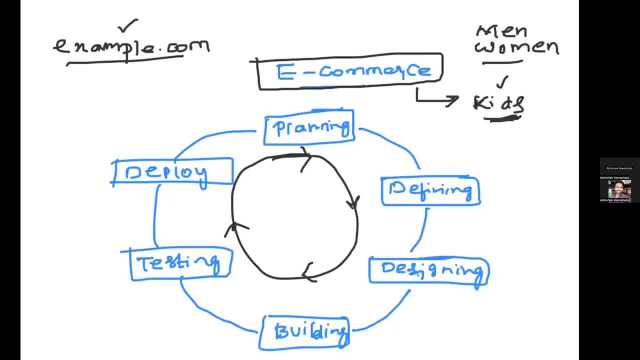 Okay, so in such cases, End of the day, It's your call, right, Because you are a devops engineer who is thinking of improving your organization's efficiency. So it's not your manager or it's not somebody else as a devops engineer. 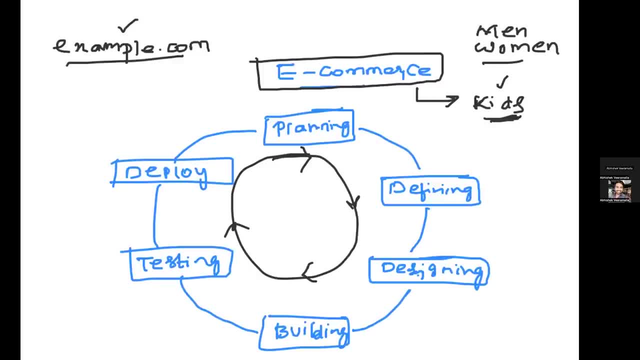 You have to suggest them that, okay, terraform might be a best tool in the community, But for our organization it's not a right fit. So think in that approach every time you work in, whether in the current organization or in your future organizations. always keep this approach. 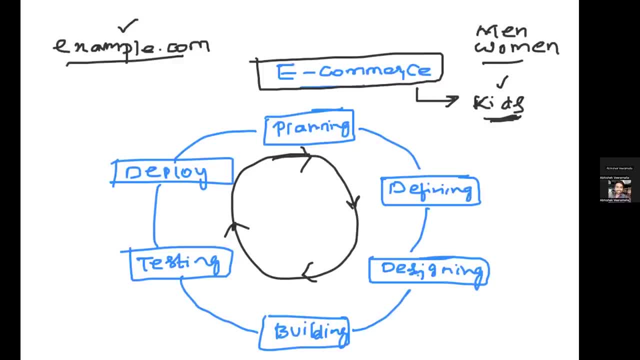 Okay. So, firstly, what happens is there is a high-level design that is decided to launch Kids catalog. So who has decided this? Let's say the organization, the CTO or somebody has thought, they just given a thought that, okay, The kids catalog might be a good option. 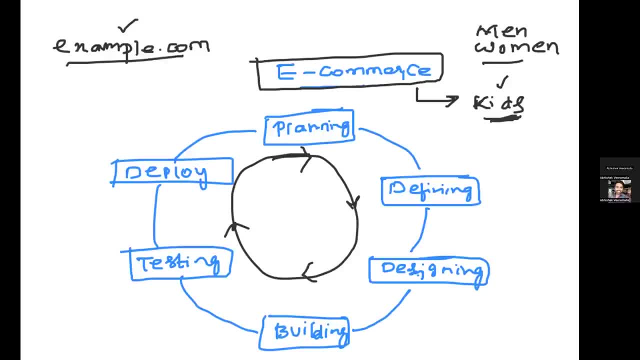 So now what happens is: once they are done with that, So you know, you will move to the planning phase. So what happens in the planning phase is you have to gather the requirements right. So as a CTO, CTO can suggest you many things, but who has to do the planning? 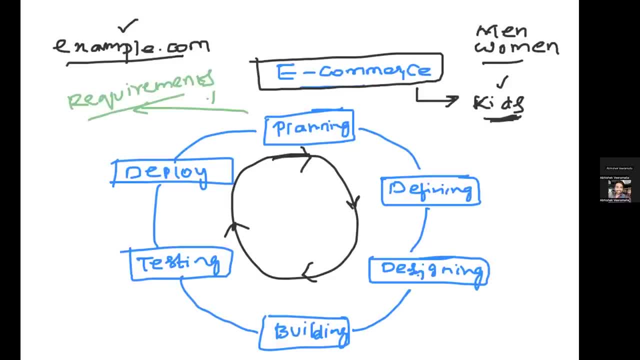 Planning and requirement. Okay, planning plus requirements. So who has to do the plannings and requirements gathering? It has to be your- I mean your- core members, right, Whether it's your business analyst or your product owner. So they have to deal with the planning plus requirement stage. 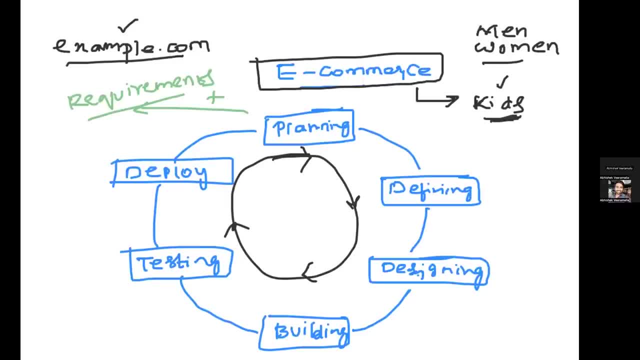 Okay, So what happens in the planning plus requirement stage? It's a one of the fundamental stages because it's a starting stage of your software development lifecycle and your product owner or your business analyst or your senior members can also get involved. You know they get the input from the customers. 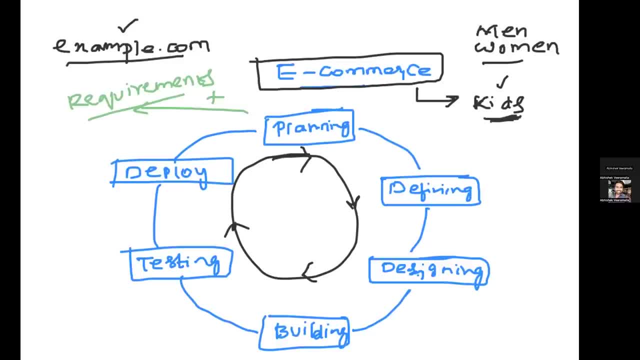 So let's say, examplecom is already live to the customers, So you have to gather your feedback from the customers. what your customers are feeling, Okay, are your customers are feeling, if you launch a kids catalog, Is it useful for them? if they are thinking, if I mean, if you have 10 customers and you are looking at potential customers, another 15-20 members and if nobody is interested in the kids catalog, then it's of no use to launch. 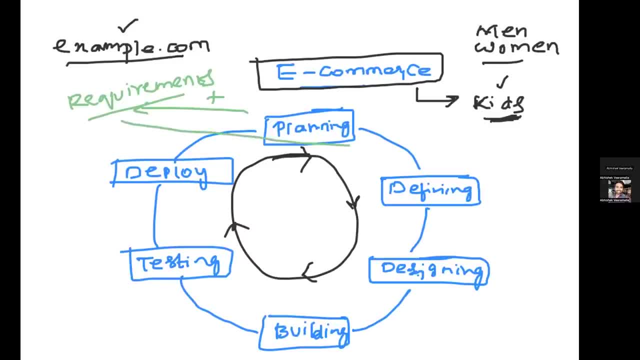 So what you can do is you can suspend the idea at this stage only. You know you do not have to propagate This idea to the all the other stages. So that's why planning and requirement is one of the most important stage. Okay, when I say requirement, what you have to do in terms of requirements, you have to gather the requirements. 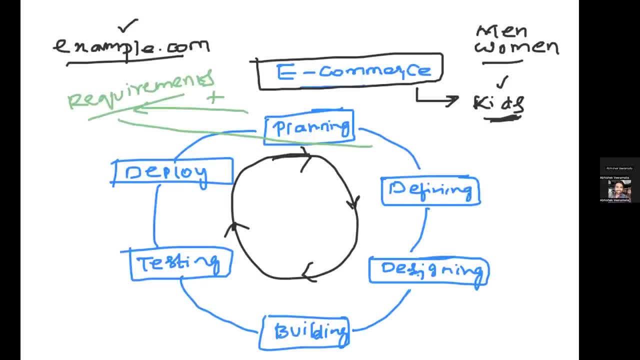 Let's say again the same example. you have 10 customers today and potential customers are 15 to 20.. What you have to do is: even in the kids. What are your customers are interested? Are they interested in the kids range between 6 to 12?? 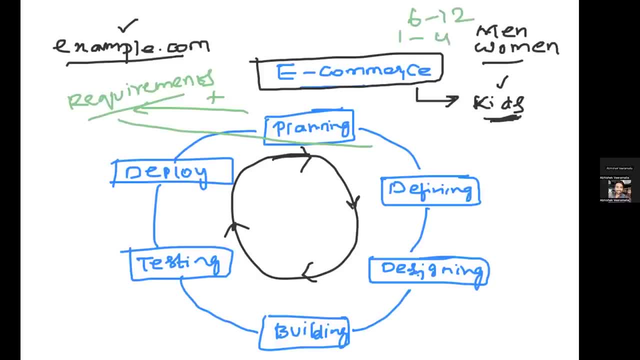 Are they interested in? the kids range from 1 to 4 years. So you have to get this information Like: how many customers Are interested in this one, How many customers are interested in this one? Once you have this collective information, that face is called planning and requirements face. 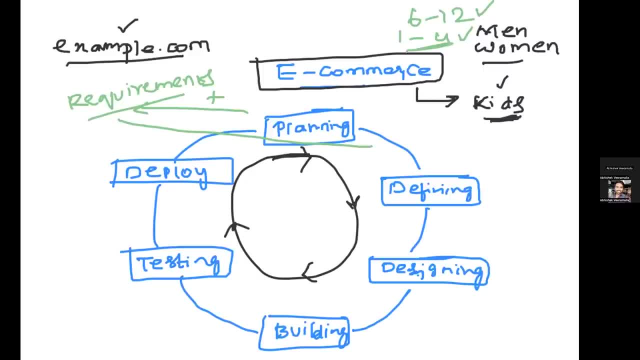 Once you come up with this planning and requirement face, then you can start with the defining and designing face. Okay, So, in terms of defining requirements, what you do is that you clearly define this requirements in terms of documents, Okay, No, What do you mean by documents? 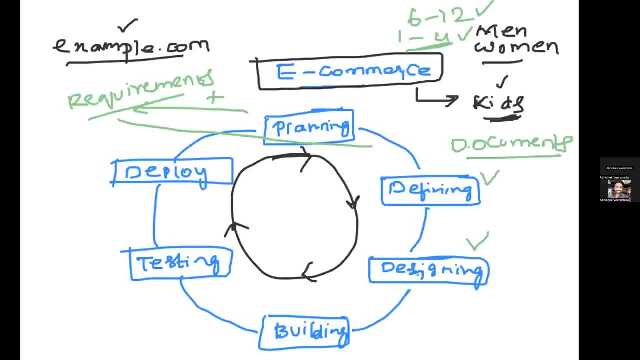 So, in terms of documents, you have to write like you know, Whether it whether, let's say, your product owner is there or your business analyst who is talking to our customers, Somebody, what they have decided is that, okay, I did a customer research and on my customer research, 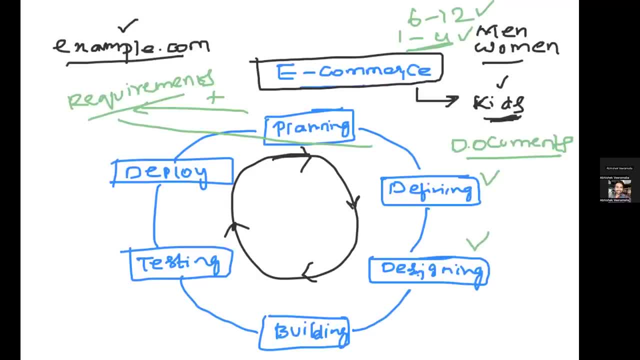 I understood that 6 to 12 years for customers are interested. 1 to 4 years- 16 customers are interested. Now what they'll do is that they will write a document that is called a software requirement specification document. Okay, So in software requirement specification document they would provide the all their data that they have collected. 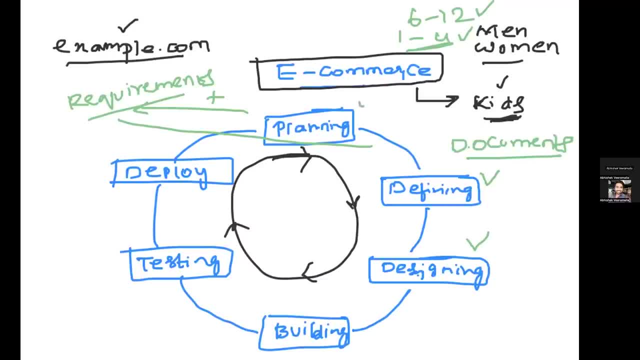 As part of the planning face. After that we will move to the designing face. Okay, So designing face is very critical face because in designing face you will do high level design and low level design. Okay, So what is high level design? HLD and LLD. 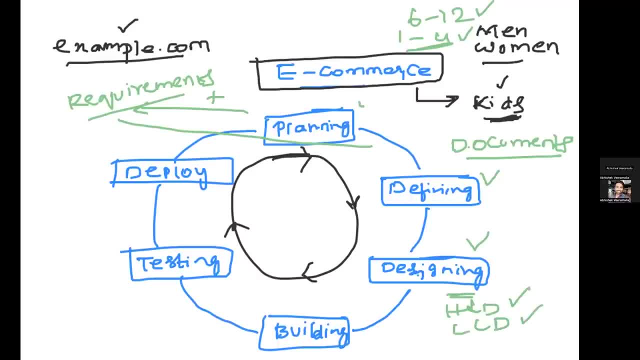 So, HLD and LLD, Let's say you have a architect, Okay, Or you have a team leader or a senior resource. What this members will do is they will write a high level design. on the high level design. You will be talking about the overall. like you know, your system has to be scalable, or whenever there is a requirement. 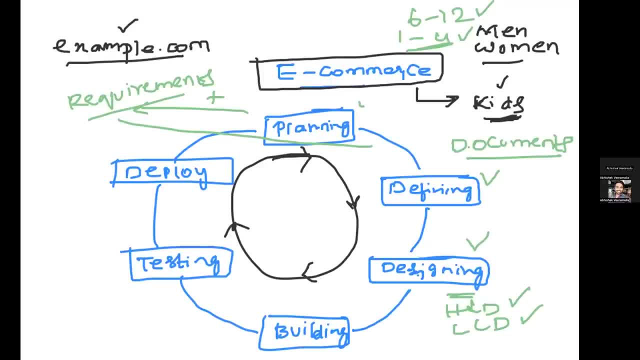 This kids catalog have to be scalable to. probably there might be more load for the kids catalog during Christmas. So you have to build your kids catalog application in such a way that it is scalable when required or it is highly available. So these things you will define in HLD. 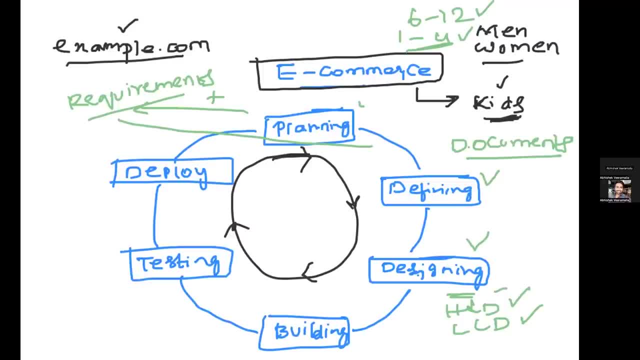 You might say that you know, I want to use this kind of database, I want to use n number of replicas, I want to use n number of replicas of my application. So such things are defined in the high level design. and coming to the low level design, your architect, or, again, your senior member of the team, the development team, 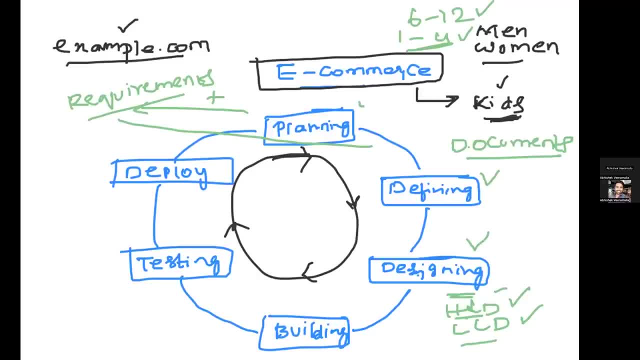 What they would do is they would write the low level design requirements. That is okay, Let's use this particular functions or let's use this particular modules. Let's say your organization is using Java or Python. So in the low level design, the senior members of the team would design, would design the systems in such a way. 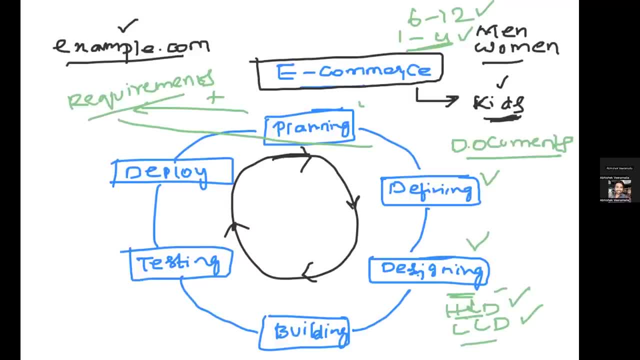 They would mention that, Okay, I want to use SQL, My skip, my SQL database. I want to call from this application. I want to make a function call. So all those these. like you know, it has to pass such an argument. 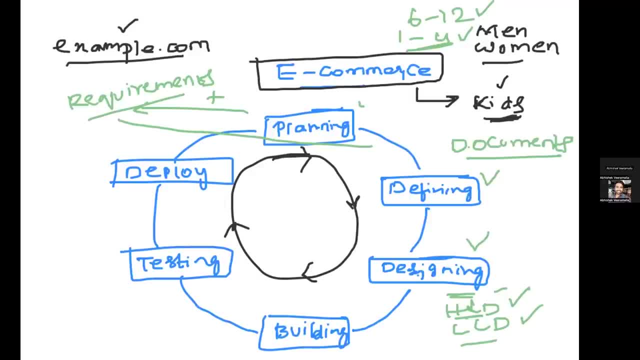 It has to receive such response. So these kind of things you would mention in the low level design that is very low, extremely low level design, Perfect. So now you understood what is planning and requirement, You understood what is defining phase, You understood what is designing phase, and then what would do is: we will move to the components that are most 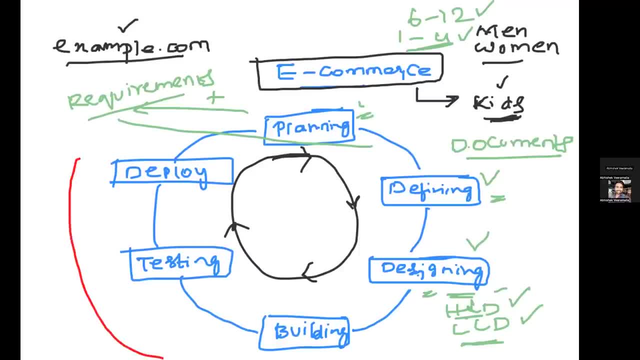 Important for devops engineers. Okay, So till this point of time, as a devops engineer, you can get involved out of your personal interest. But where your actual importance would come into picture is these three phases, that is, building the software, testing the software and deploying the software, and as a devops engineer, you can automate this processes. 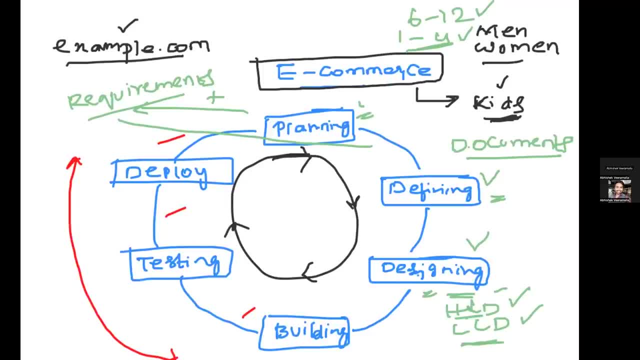 Okay, So our focus of interest always is automation. So that's why here you can bring in your automation. So which phases of software development lifecycle are devops centric or or a devops engineer should be interested in? that are building phase, testing phase and deployment phase. 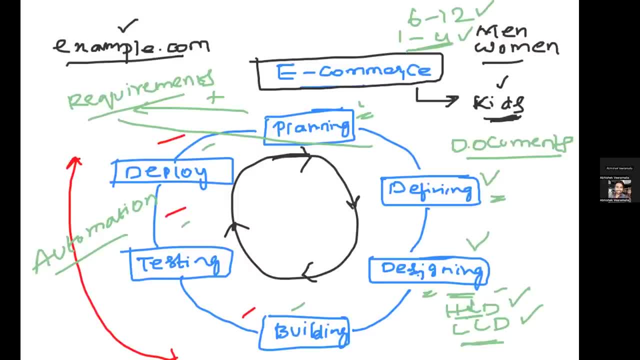 No, I'm not saying that you should not get involved in the designing, defining or the planning phase. Let's say you are a critical resource of your team or you are a devops engineer who is development in heart. Okay, Probably you are also interested in development and devops engineer in such cases. 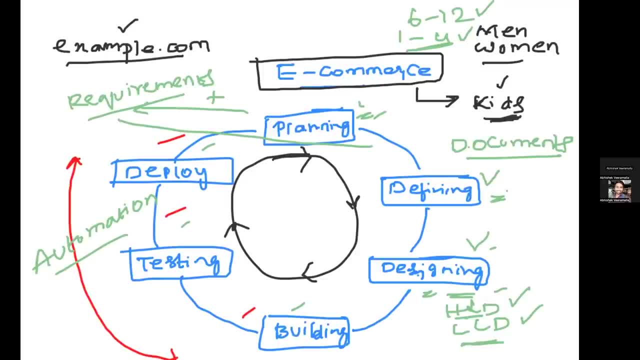 You can get involved in all of these phases, But primarily as a devops engineer, your point of interest or your focus of interest should always be these three things, that is, building a software, testing a software and deploying the software. So what I'll do is we'll take these three phases in the next slide and we'll try to understand each of them in detailed. 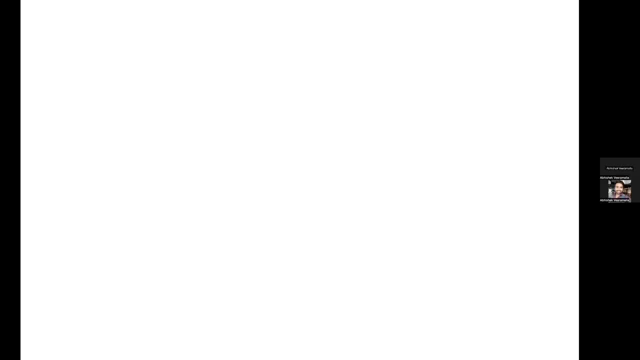 Okay, We'll come back to this slide again, But before that, let's try to understand these phases in detail. that is Building, Then you have Testing and finally you have deployment. Okay, So these are the three phases: building phase, testing phase and deployment phase. 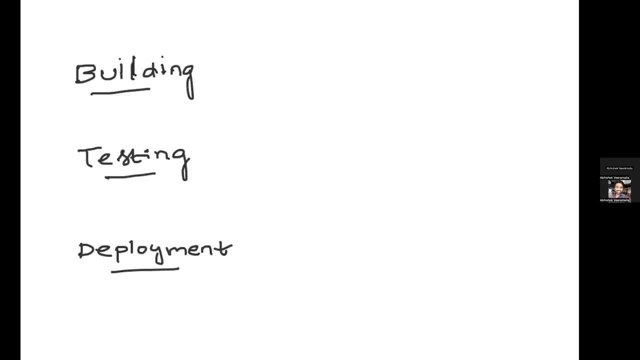 Let's try to understand each of them in detail. and how can develop, How can a devops engineer can improve the efficiency of these phases? We'll also take a look at that. Okay, First of all, building the software. What do my, what do I mean by building? 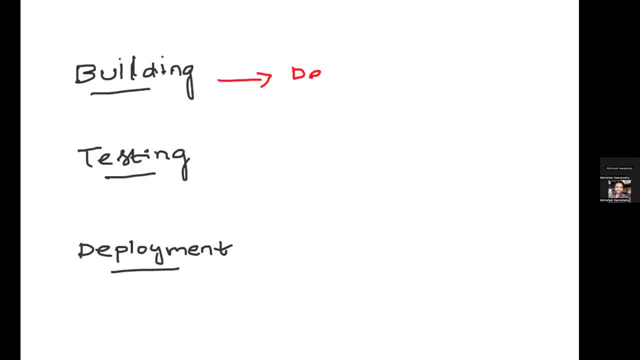 So in this case, building is nothing but developing. Okay, So once your senior members of the team have come up with the low-level design and the high-level design, let's say, and your product owner and business analysts have come up with the planning requirements and software requirement document, 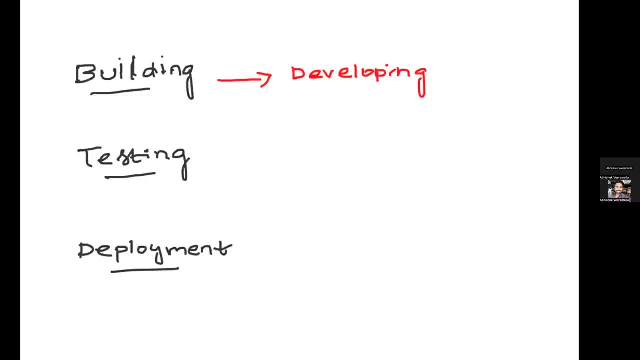 Okay, What is the next thing that you have to do Is this application has to be developed Right. So all your stories are created, All the documents are written. Now you have to move to the next stage. that is, developing Right. 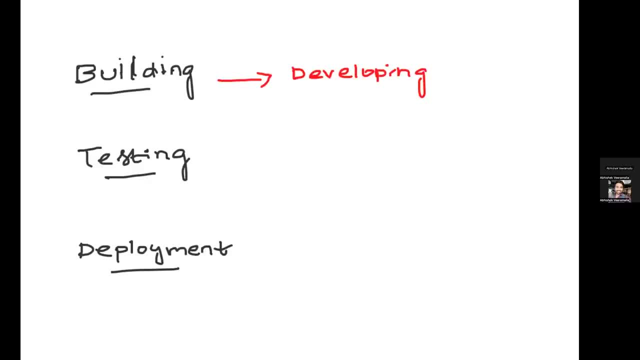 So, okay, All the things are done. You spoke to the customers, You got all the requirements, Your design documents are ready. So it comes to the developers and what this developers will do. They'll start writing the application code in their favorite language or the language that is used within your organization. 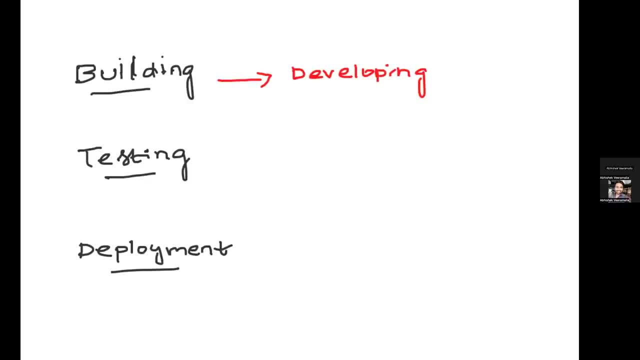 So this phase is called as developing phase. So what happens in the developing phase? Probably the custom- sorry, your developer. He will read the Jira items or he will read the documents that are prepared and he'll start writing the code. Okay, So let's say he start writing the code and what he'll do is, once he writes the code, he'll push this to a common location in the organization. 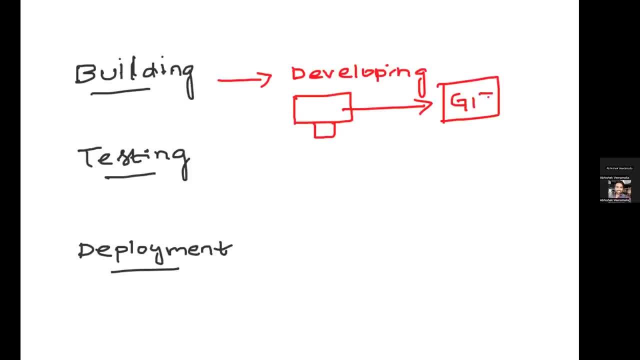 So most of the organizations these days use git. If you don't know about git, don't worry. We'll talk about git in the future, But for now just understand it's as a source code repository, That is, a repository that is storing all the code. 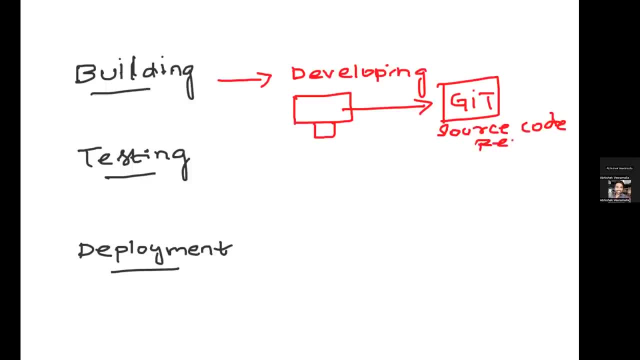 Why you need a source code repository? because it cannot be only with this one developer right. So this develop, this is a developer laptop, but you have to always share this code within the other members of the team, So that's why you store them in a source code repository. 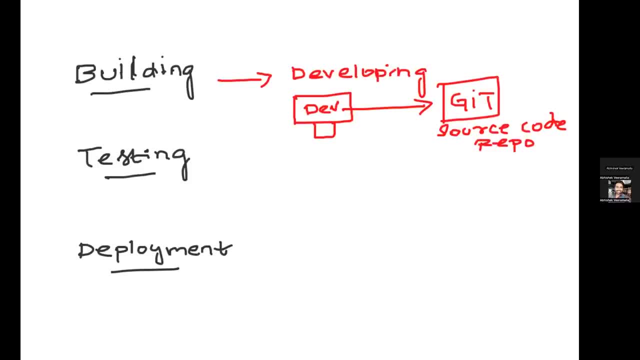 That is, a centralized repository or a distributed repository. So, for example, in this case I choose git. So now the developer wrote the code, He got it reviewed by his PR members- Okay, So PR members are nothing but other members of the team- and finally push the code to the git. 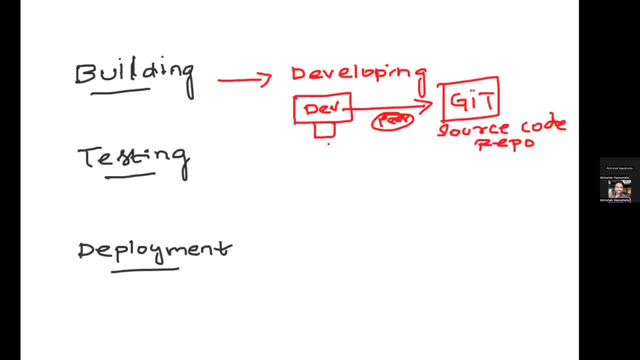 Okay, Now this is done, This phase is called as a developing phase. Once this is done, what you have to do, the next phase would be testing this application. right? So let's say? developer said that it is working fine on my server. 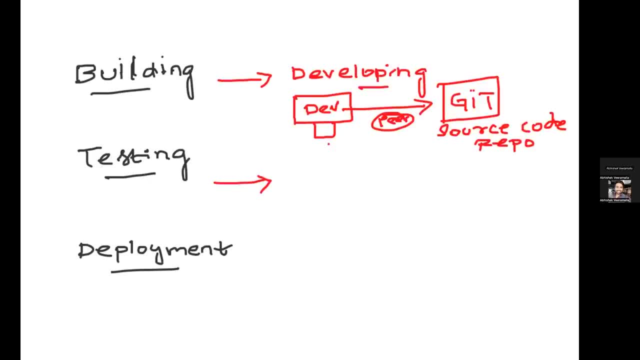 Would everybody believe it? No, End goal has to be to deliver a prompt and a quality code to the customer. So that's why it has to go to the testing phase. So this phase is called Testing phase. So what happens in the testing phase? 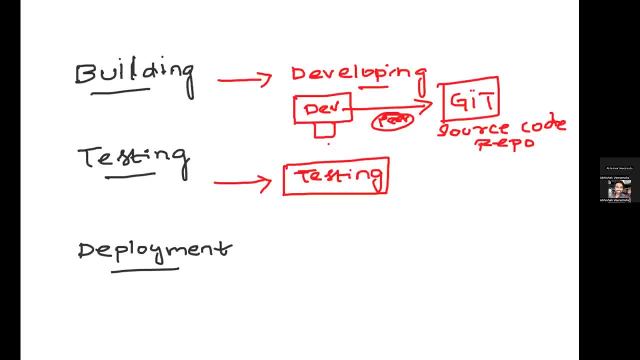 This application that is stored in the git repository, that is taken and deployed in a server, And then you have a team in the organization that is called QE team. Who are this QE team? They are the quality assurance engineers. Okay So, quality assurance engineers. 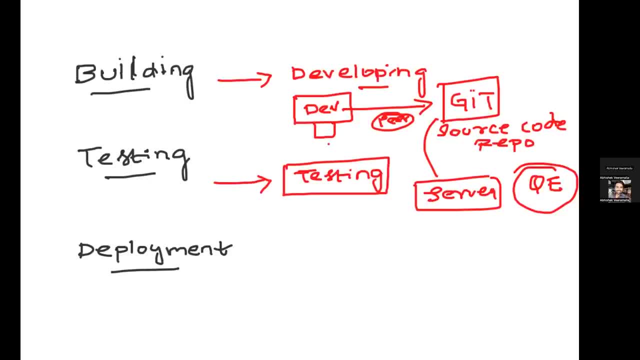 They basically take care of testing the software. So here the developers has built the software, QE has tested the software. Okay, So this phase is primarily for developers, This phase is primarily for QE engineers. And then there is a deployment phase. What happens in the deployment phase? 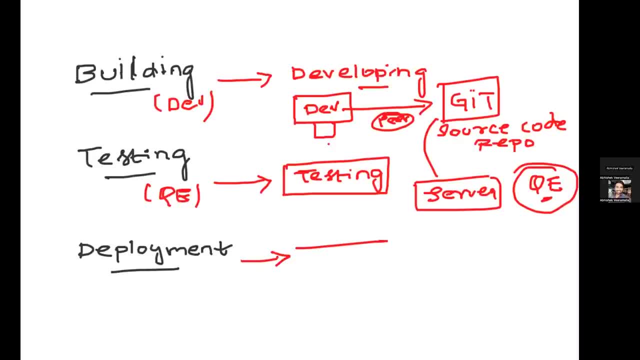 You know, on the deployment: in the deployment phase you basically Promote this application to the production. Okay, So here you are testing in a virtual server that can be, you know, Like any staging server or your development server or anything. 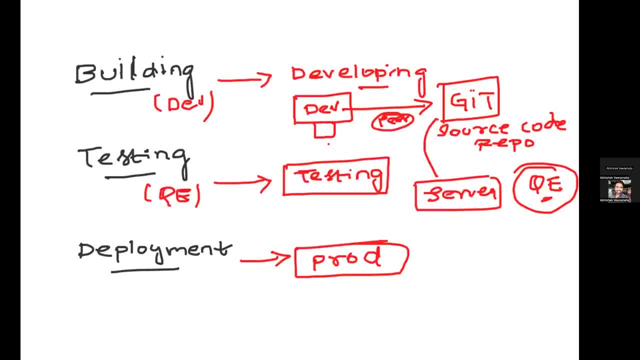 But finally you push it to a production server. right, Who is receiving this in the production server? Your customer. So this happens with the. this is the entire things that happen in a software development lifecycle. Now you have to ask me: Okay, 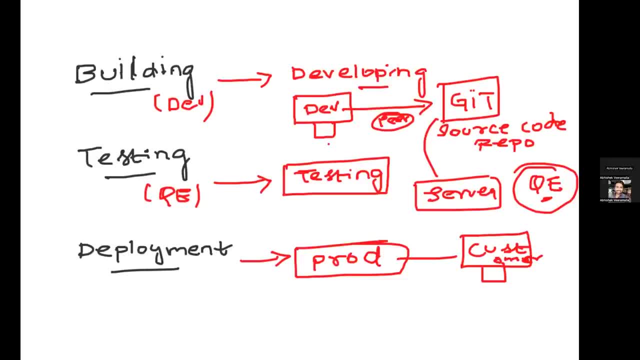 I learned about everything you said. This is used by developers, This is used by QE. Now, where is devops coming into picture? So all these three things, Okay, Even if you remember in our last class what we thought. What we learned in the last class is that 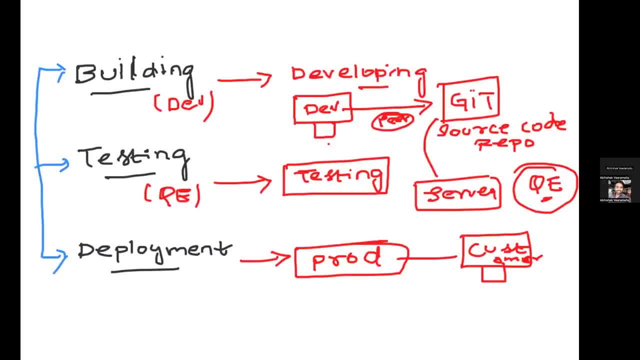 A devops is nothing, but it's just a culture, Okay. So where devops comes into picture is improving the organization's efficiency. Now, Developer has written the code. He stored it in his local repository, Okay, And finally he pushed it to the git repository. 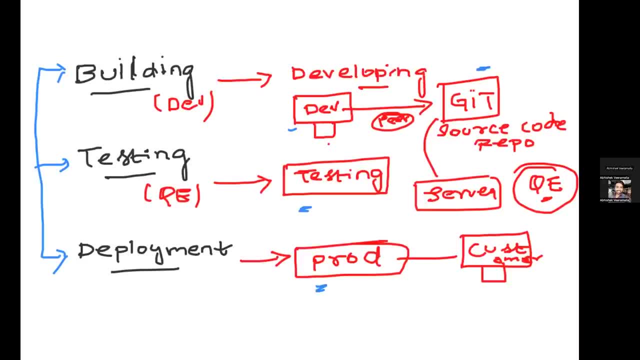 Here the testers are testing the code And here you are moving the application to the production. So devops engineer basically Fastens this process right, So he improves the process To deliver the code Quickly. Okay, And by ensuring all of these terms are matched. 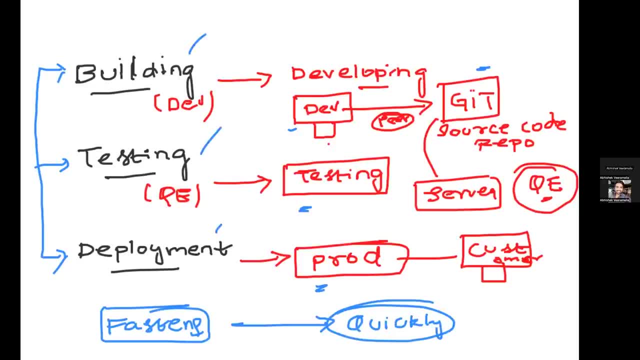 Okay, It devops. engineer ensures that the building, testing and the deployment processes are followed without any manual intervention. That is, everything happens in a automated way. Okay, So everything is automated. This is all Efficiency, Right. Just a second. Is there any problem with my speakers? 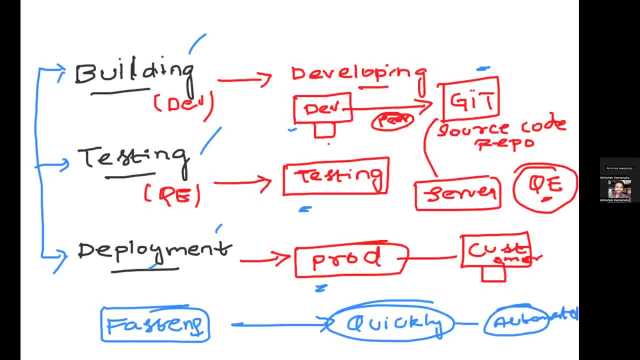 Okay, I'm not sure if the last sentence was overheard or I see some error with the speaker, but just to repeat. So what a devops engineer does? he fastens the process. Okay, By fastening the process he means that devops engineer would automate the process. 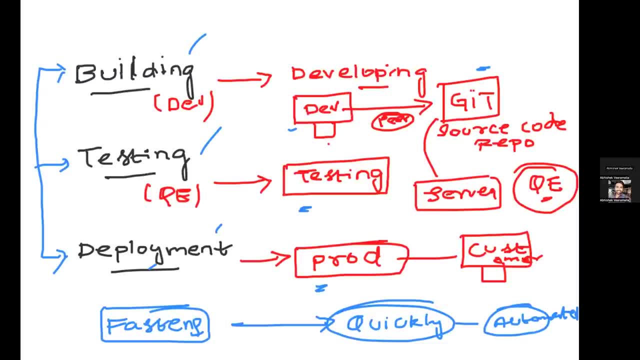 Okay, What happens with automation is that devops engineer automatically automates the process and the process. Okay, So this is the process that devops engineer needs to do, Right? So what does devops engineer do? He needs to do is: 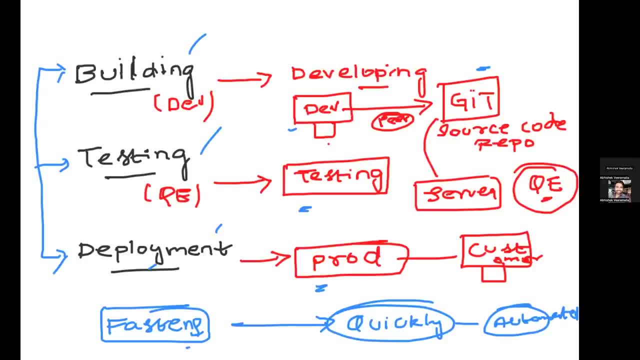 He needs to call a developer. Okay. So what does devops engineer do? He needs to call a developer. He needs to call a developer, Okay. Okay, that devops engineer would automate the process. okay, what happens with automation? always, automation will lead to efficiency, right? if you are doing a very good automation, it is always directly. 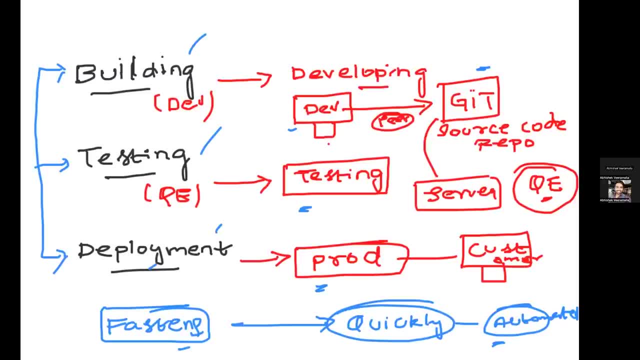 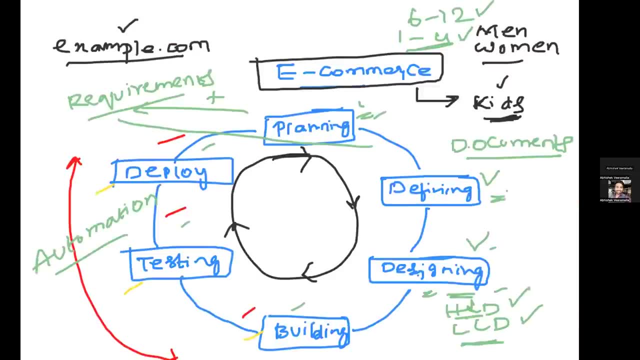 proportional to the efficiency of your product delivery. so that's why devops engineer comes into the picture. so you know, if we go back to this specific slide, a devops engineer is primarily responsible for automating these three phases of your software development lifecycle. so that's why. 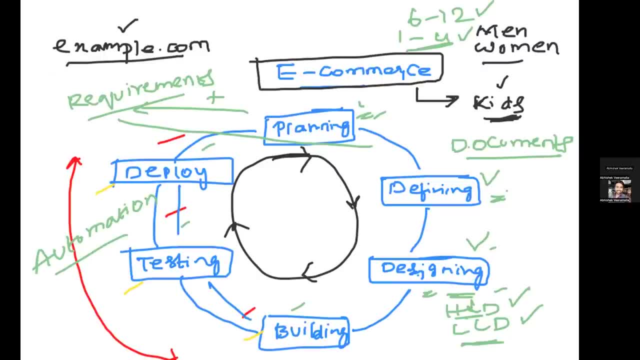 it is very important and essential for everybody to understand software development lifecycle, whether you are a devops engineer, a developer tester or anyone. because in an organization, you all work together. right, when you are working together as a team, you have to follow a certain standard. so that standard is called software development lifecycle. and because we are focused 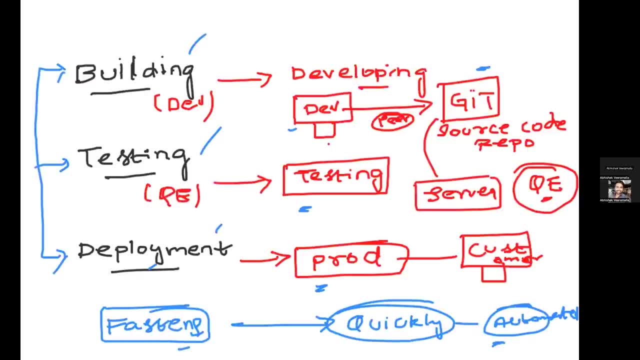 in devops and because we are learning devops in these classes, you have to understand that a devops engineer is primarily focused in building, testing, deployment, automation right. so devops engineer is not individually involved in building because he does not develop the software, he does not test the software, he does not deploy the software. 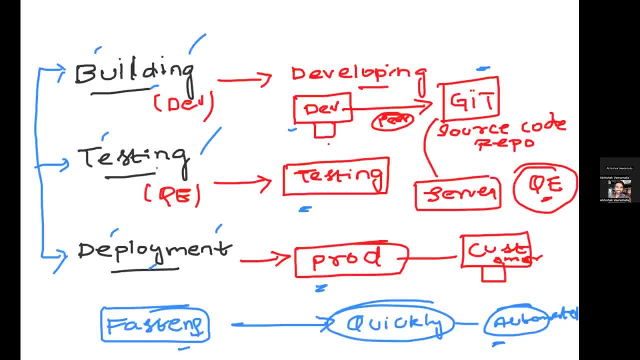 everything happens automatically, right? so manually, you are not going to deploy this software in production, so you are going to, as a devops engineer, you are going to automate and write this automation scripts so that it improves the efficiency and reduces the time by avoiding manual intervention. so now i hope. 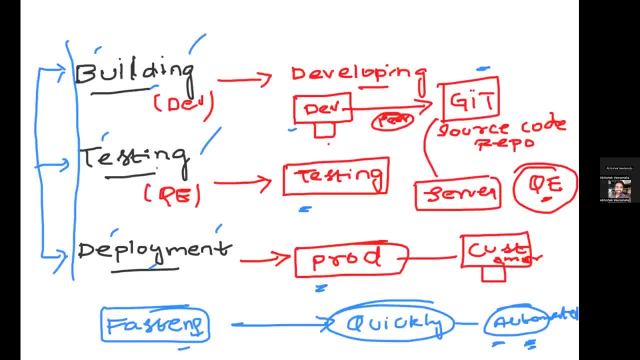 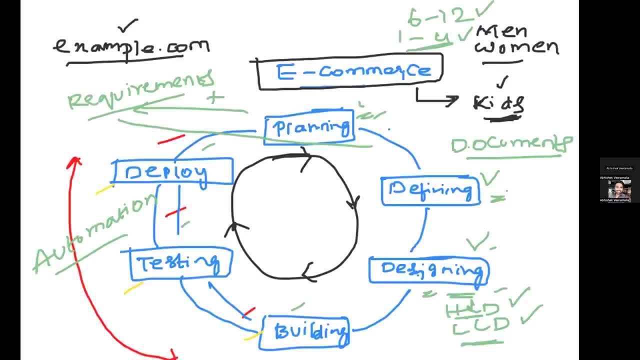 gown software development lifecycle is clear to you. and finally, if we go back to this slide, you know all this process can be done in different ways. okay, so if we are talking about the project management, there are different things, like there is a waterfall model, there is iterative model. 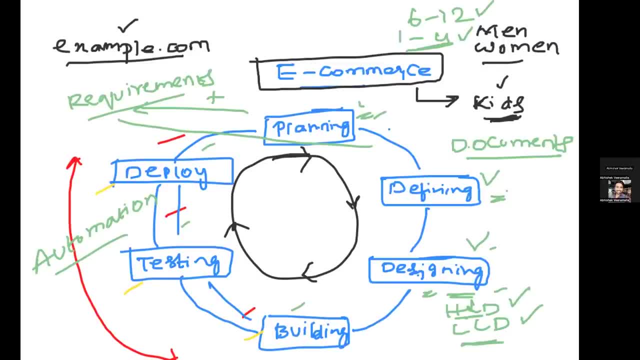 there is agile model. so what are, what are these models? we learn during our project management classes. so there is a project management class, but on a high level. you have to understand that every organization these days is using a agile methodology. so in agile methodology, what has the AI low brand? 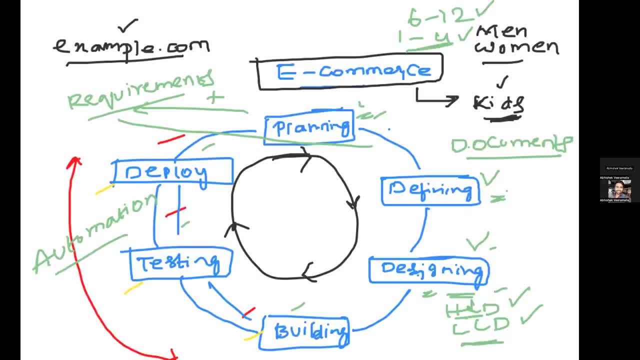 definition you have to understand is that every organization these days is using an agile methodology. so in agile methodology, what happens is you follow all of these phases, but you do it agile, like you know. you take short sprints, that is, you don't wait till all of your planning is done, or 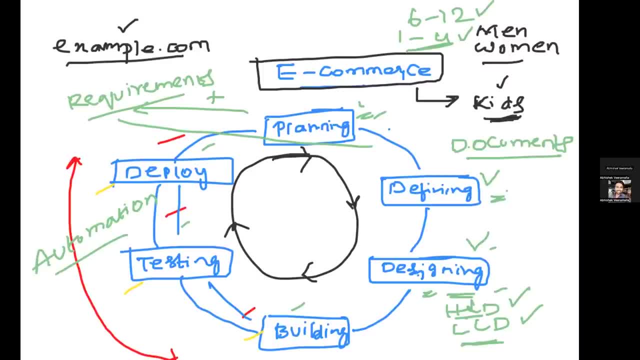 you don't wait. all of your define or design documents is done. once a small chunk of it is done, you start with all of this process and then the other chunk is done. you again follow this entire circuit that is called agile. but we are not going into depth of these concepts at this. 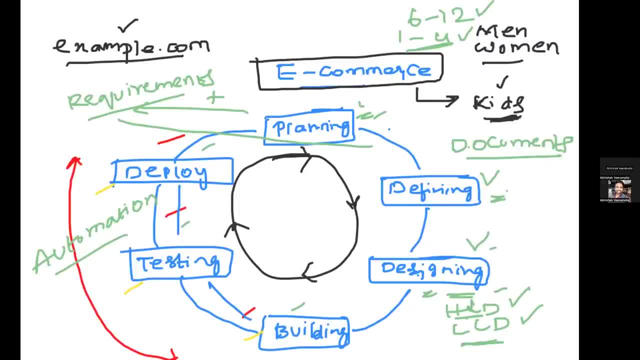 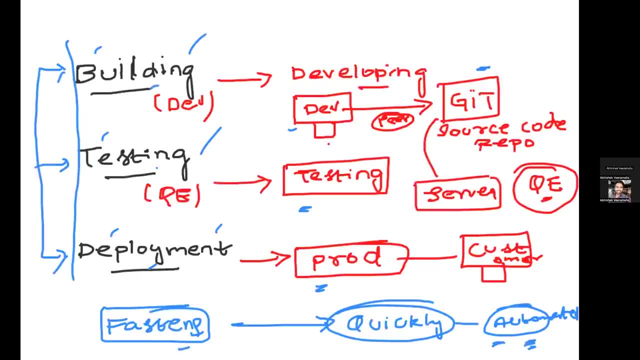 point of time. so the primary idea of this class is: everybody should understand the concept of software development lifecycle and how devops engineers are important for the software development lifecycle. okay, i hope it is clear and if tomorrow in any interview questions, if somebody is asking you what are the pillars of software development lifecycle? and, as a devops,